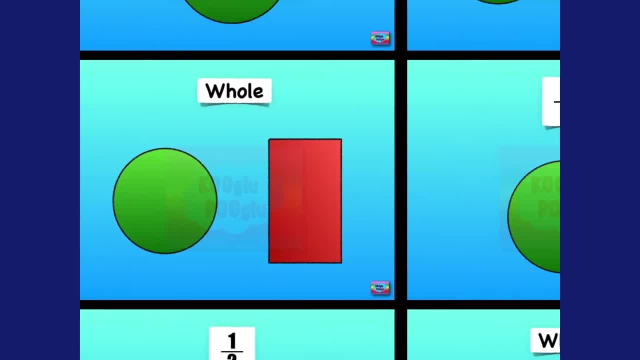 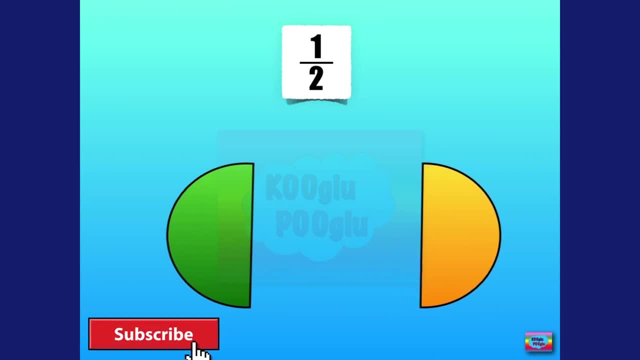 all divided into pieces. Here is a half. A half is from one whole. you divide it into two parts. Here we have another example of a half, but with a rectangle. Just like I said, if you're doing a half, one whole is divided into two parts. Here we have. 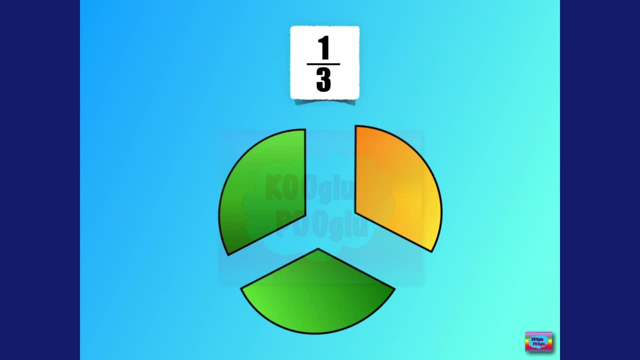 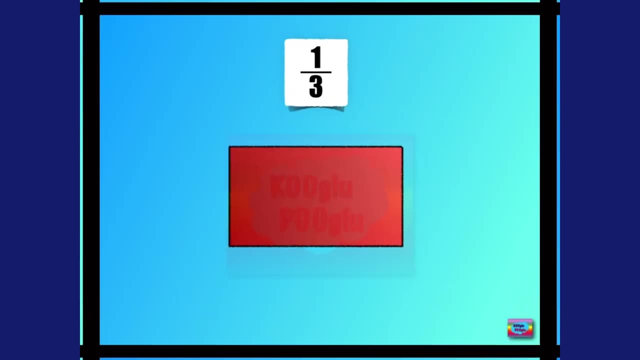 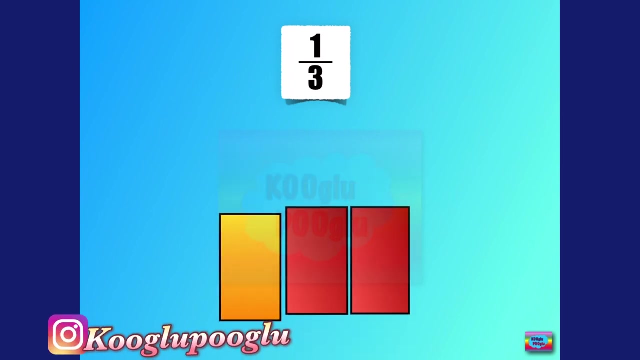 one third. This means that one whole is divided into three parts. So all of them are cut into one third, but the orange one represents that one of them are shaded and the other is not Same thing. over here Only one part is shaded in, but all of them are one thirds. 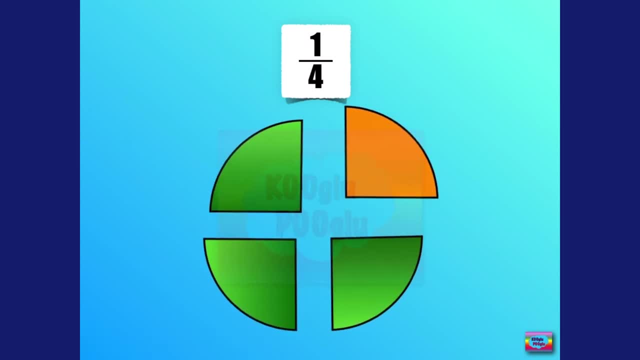 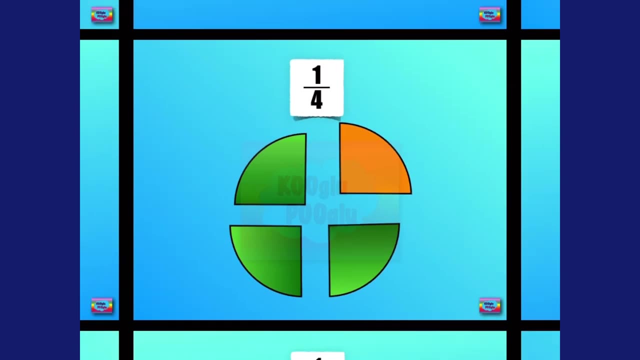 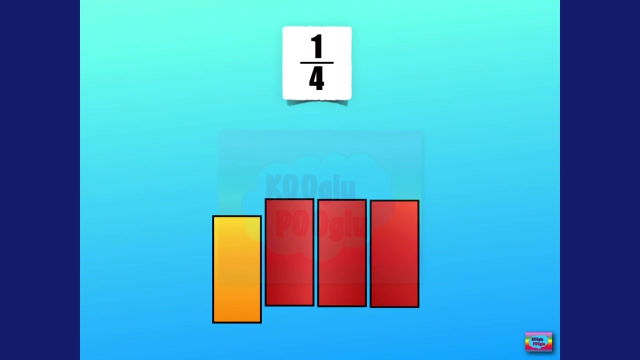 Here we have now one fourth. This means that a whole is divided into four parts, And the fun fact is, did you guys know that one fourth is called a quarter? Here we have one fifth. As you can see, here all of them are one fifth, but one is shaded. 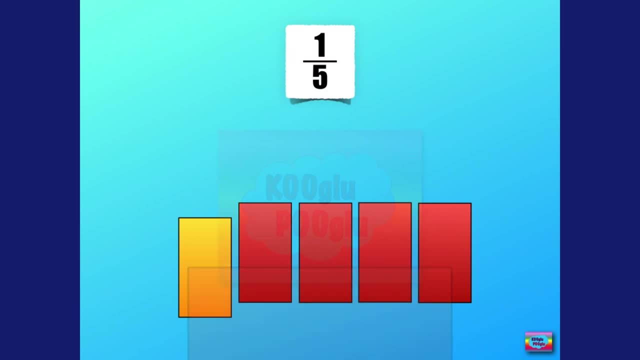 Just like over here, it shows that it's cut into a bunch of pieces. Hey, this kind of reminds me of something. This reminds me of cutting up a chili pepper. and then there's that one yellow part. Here we have one third. 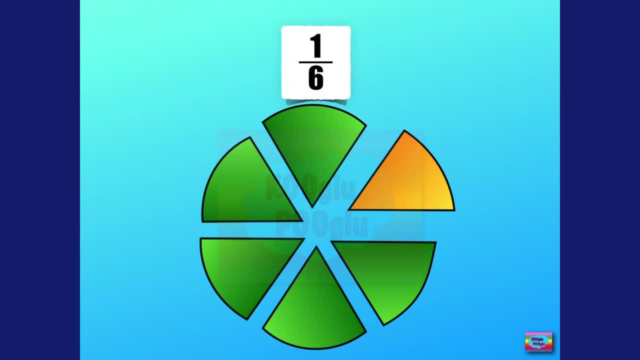 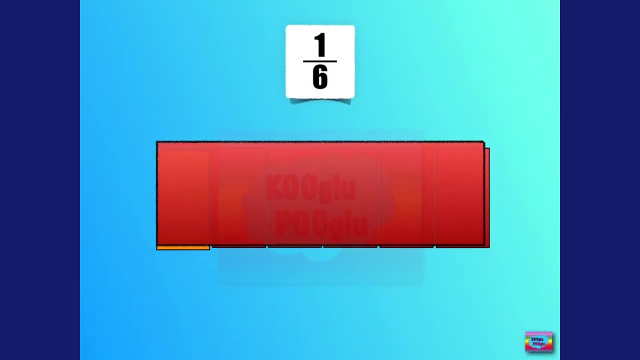 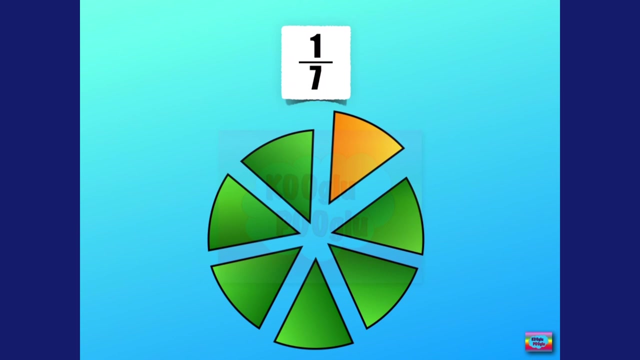 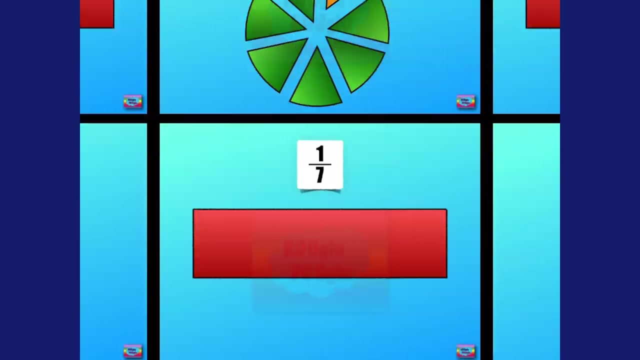 sixth: oh, this looks like a pizza and here every part is a one. six: that means one whole is divided into six parts. again, chopping up the chilies, here we have one. seventh: this means one whole has been divided into seven parts, equal parts, to be specific. chop, chop, chop, chop, chop.